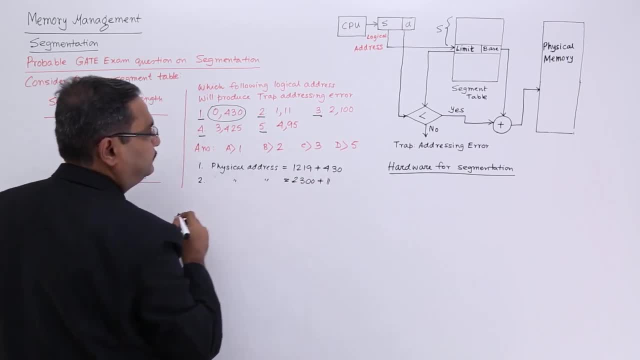 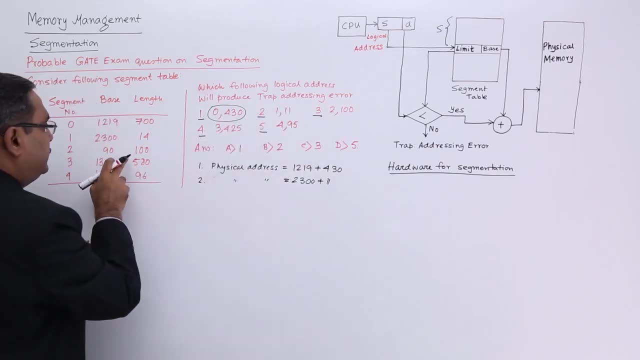 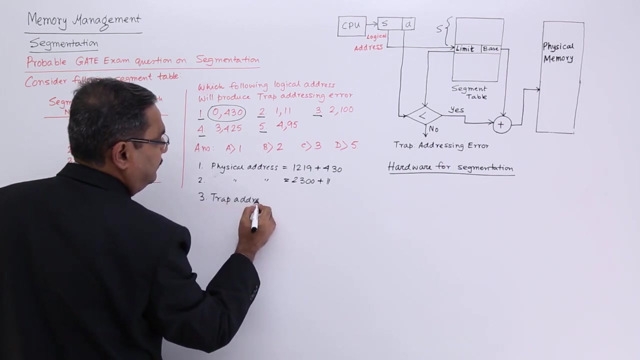 2300 plus 11.. 2300 plus 11.. Next one: 3, 2, 100.. You see, 100 is less than 100 is false. This is it will produce a logical error. So that is a trap addressing error, Because 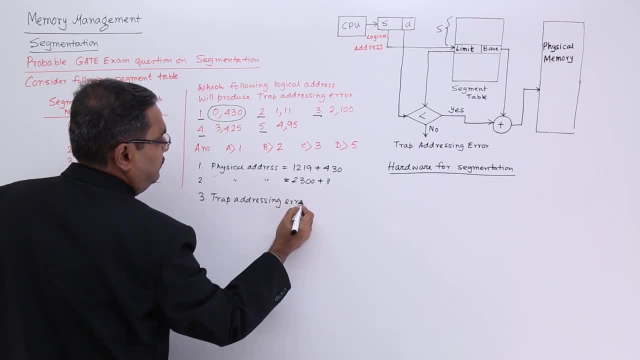 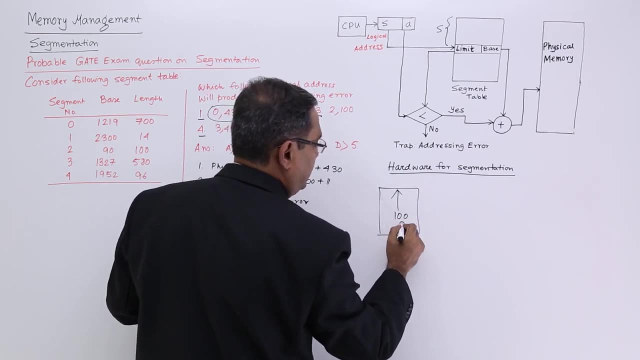 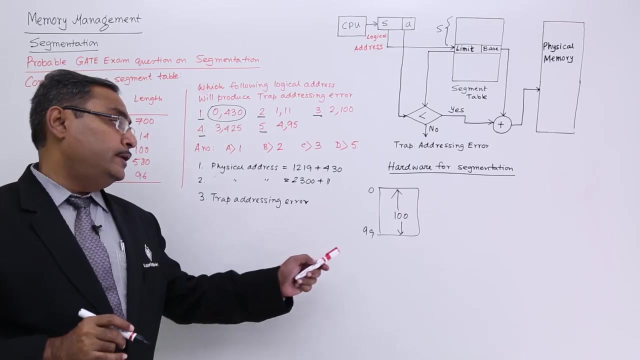 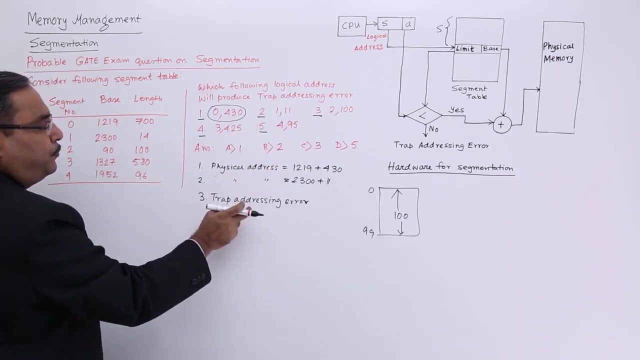 I told you this one earlier. A program may have 100 bytes, but its address will be ranging from 0 to 99. The offset address will be ranging from 0 to 99. So this 99 must be less than the size of the program, at least 1 less than So. that is why, as they are equal, so it will. 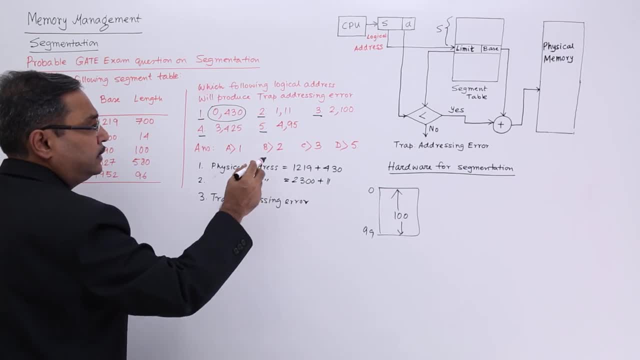 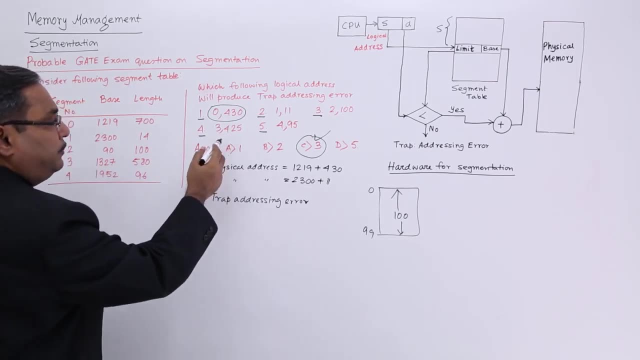 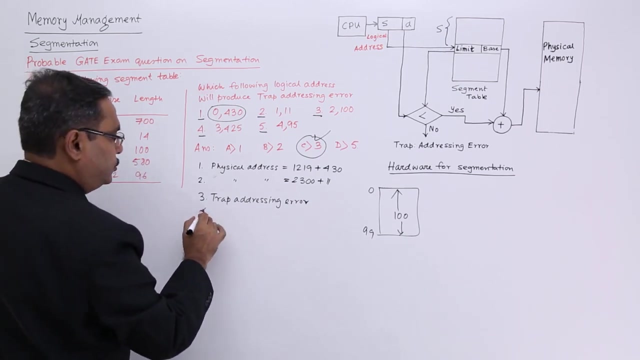 produce a trap addressing error. So physical address cannot be calculated. So 3 is the answer. So this is the answer. So C is my answer. in that case, Let me go for the other one: 3, 4, 2, 5.. So 3, 4, 2, 4, 2, 5 is less than 5, 8, 0. So it is okay So. 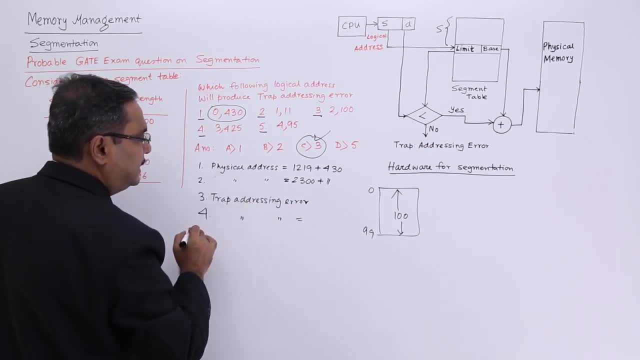 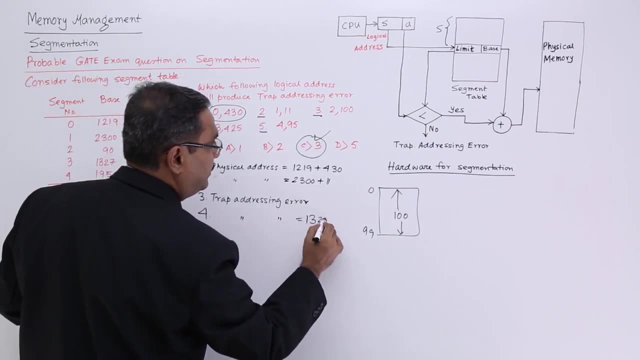 4.. That is a physical address. Do not consider this one. That is a physical address, And then it will be 1327.. 1327 plus 425.. And the last one: 3, 4, 2, 5.. So 3, 4, 2, 5.. 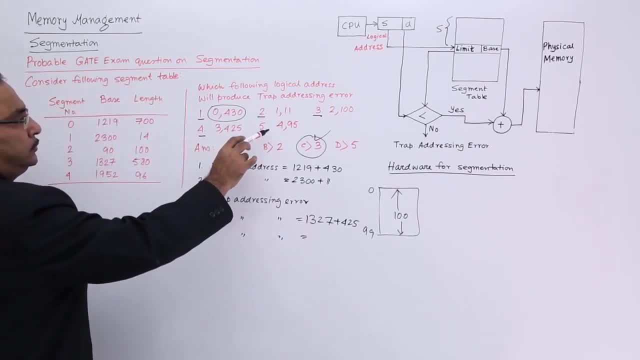 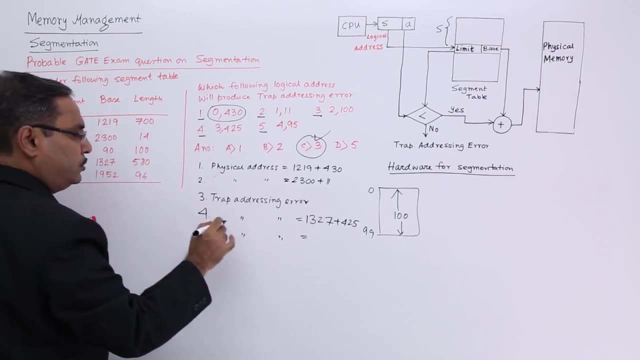 Physical address: 95.. 95 is less than 96. Just it is 95. So 95 is okay. So physical address will be 1952 plus 95. So whatever the value you are getting after doing the, 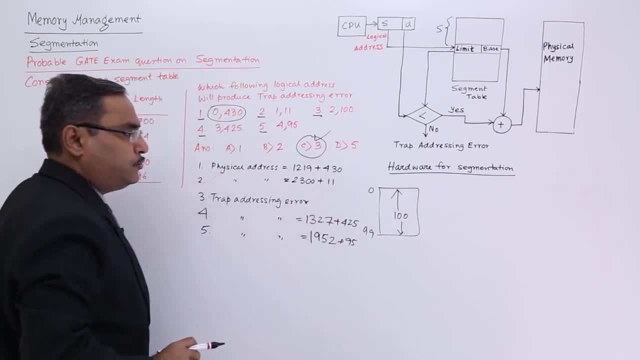 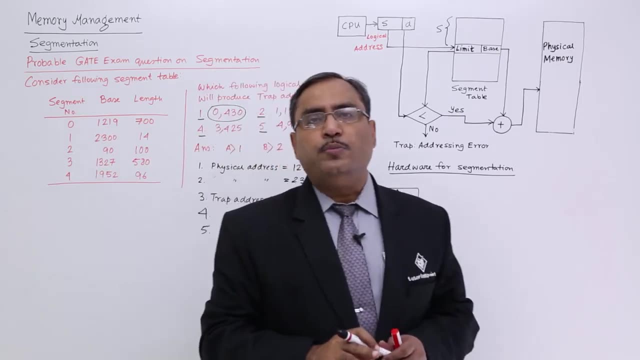 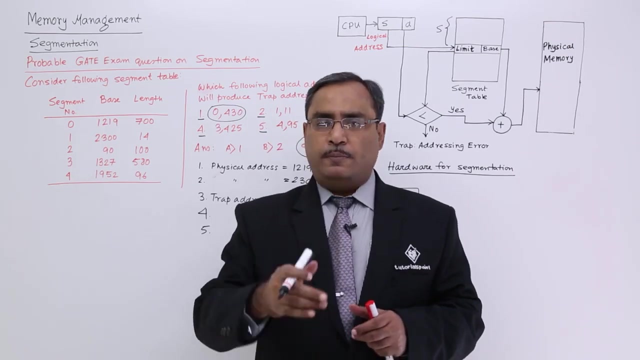 sum, you should have to work accordingly. So in this way, the problem has been answered. This question has been answered. So in this way, if you get such numerical problems, do not leave these opportunities, Because these problems will carry marks for you. Thanks for watching this video, Please. 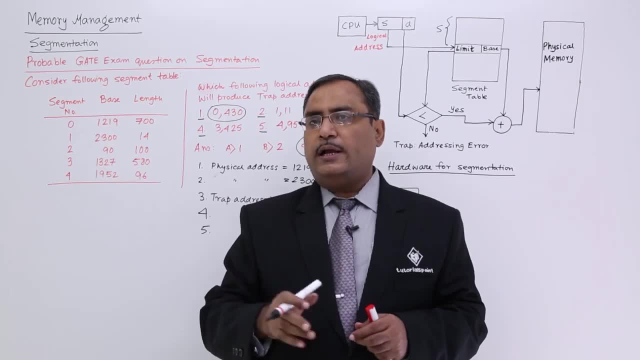 wait for other videos coming on this particular memory management and other topics. Probable get questions will be there. Please watch them, Thank you.